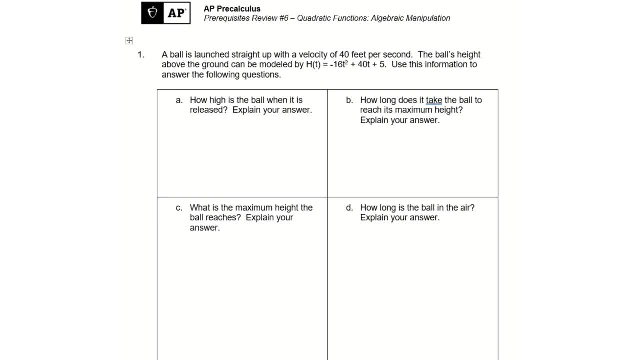 that have gone by right. So part a asks us how high is the ball when it is released? We're being asked how high, so we're being asked to find the height. That must mean that when it is released tells me an amount of time. When it's released, no time has passed, so that means time equals zero. 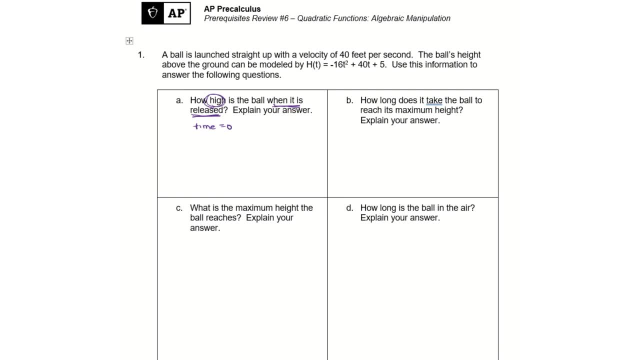 So if we just plug zero in for t, substitute zero for t, we're going to have negative 16 times zero, Zero squared plus 40 times zero plus five, which means that the ball is at a height of five feet when it's released because no time has passed. 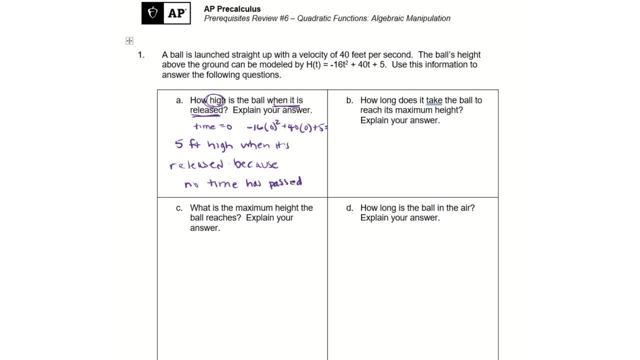 All right on to part b: How long does a ball last? How long does it take the ball to reach its maximum height? And part c: what is the maximum height the ball reaches When we see the word maximum or when we see the word minimum in a? 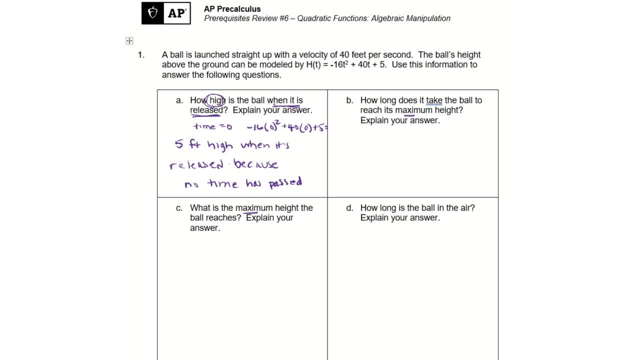 problem like this, we should immediately be thinking about the vertex on the graph. So both of these are asking us about the vertex. How is that possible? Well, that's possible because the vertex is a single point, and a point has two values. right, It has an x-coordinate and a y-coordinate. 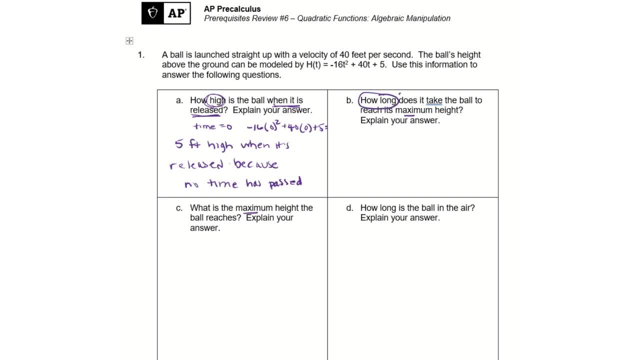 So in part b we're being asked: how long does it take? That's time. And in part c we're being asked for the maximum height. So in part b we're being asked for the x-coordinate of the vertex. 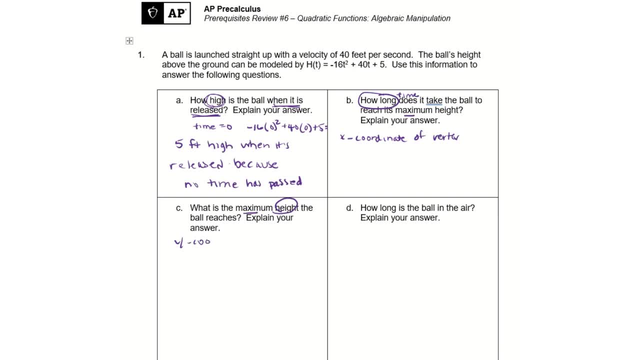 And in part c we're being asked for the y-coordinate of the vertex, So to find the x-coordinate of the vertex. when we did our review we were asked to find the y-coordinate of the vertex. So in our review lesson I reminded you that that's negative b over 2 times a, or in this case, negative 40 divided by 2 times negative 16,. 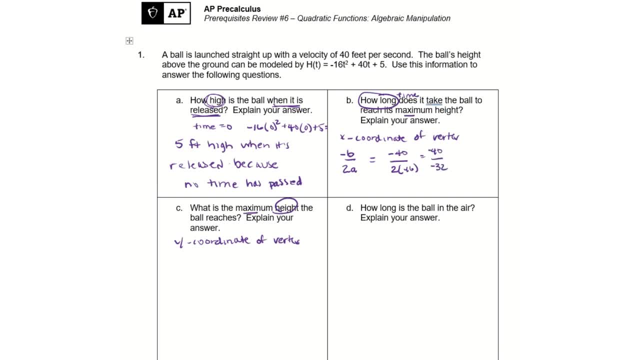 which is negative 40 over negative 32,, which is 1.25 seconds. Now I need to go find the y-coordinate of the vertex. next, If I know what the x-coordinate is, I need to just use the x-coordinate. 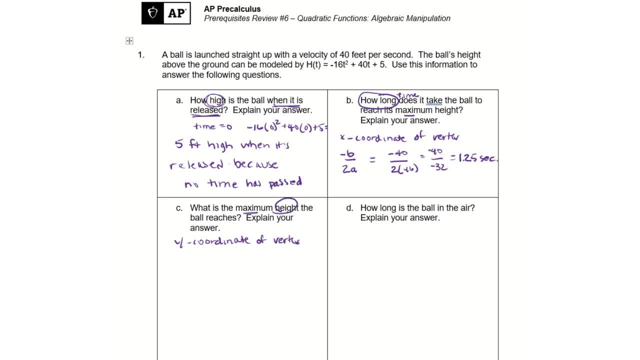 So I need to take the y-coordinate over 1 cambio and I'm going to use the ganonghit- excuse me, I'm going to closet it in place of the y-coordinate in order to calculate the y-coordinate. So I'm going to take 1.25 and I'm going to substitute it in place of t because danced. 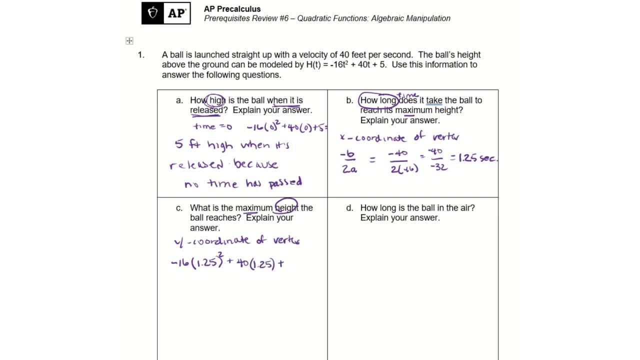 it's 1.25 seconds, So negative 16 times 1.25 squared. 1.25 squared plus 40 times 1.25 plus 5.. Minus 15.. 40 times 1.25 is 50 and negative 25 plus 50 plus 5 is a maximum height of 30 feet. 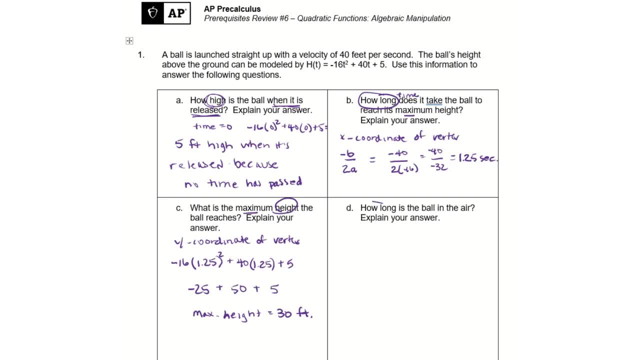 part d says: how long is the ball in the air? how long is seconds right? i'm being asked to find seconds. that must mean that the how long is the ball in the air tells me the height. well, if the ball's not in the air anymore, then it has to have hit the ground, and if it has to have hit the 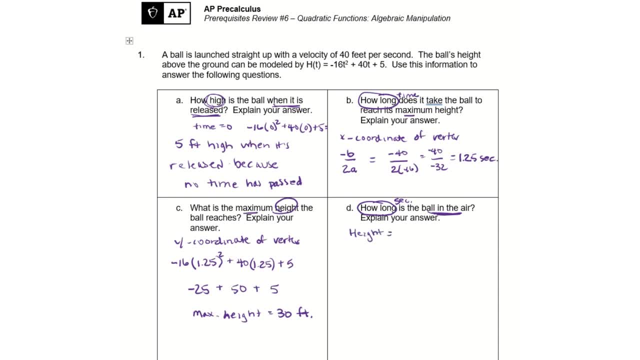 ground, then that means that we're talking about a point in time where the height equals zero. so we're going to substitute 0 in place of h of t. 0 equals negative 16 t squared plus 40 t plus 5.. to solve this, we're going to need to. 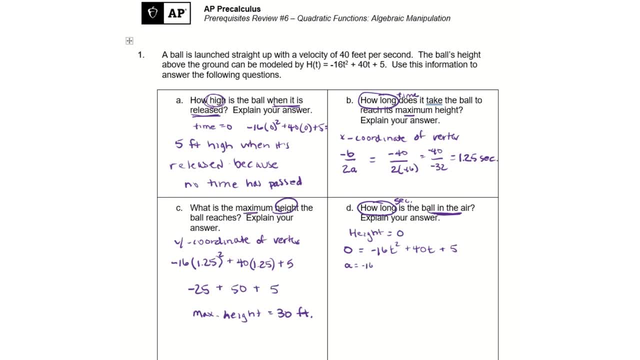 use the quadratic formula. a is negative 16, b is 40 and c is 5.. when i substitute those numbers into the quadratic formula, i have the opposite of b, which is negative, 40 plus or minus the square root of b squared. so 40 squared minus, 4 times a, which is negative, 16 times c, which is 5. 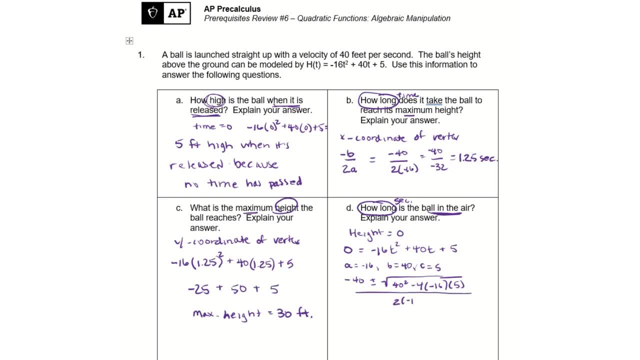 all divided by 2 times a, which is negative 16.. next i'm going to simplify what's under the square root. so i get negative 40, plus or minus the square root of 1920, all divided by negative 32. now when i take the square root of 1920, it comes out to 43, point something. 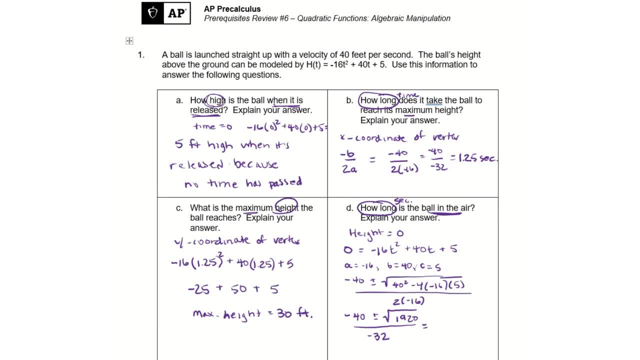 43.18. negative 40 plus, that value is going to be positive, and a positive divided by a negative 32 would give me a negative answer. i can't have negative seconds, so i'm going to ignore that answer and i'm going to focus on negative 40 minus the square root of 1920.. when i do negative 40, 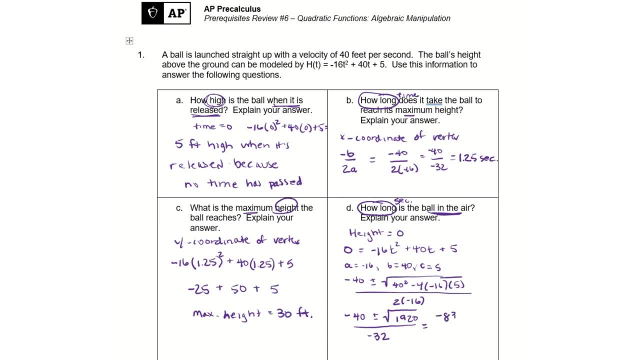 minus the square root of 1920, i get negative eighty three point eight two divided by negative thirty two, and when i divide that i end up with a final answer of 2.62 seconds. the ball is in the air for 2.62 seconds or the ball hits the ground after 2.62 seconds. okay. number two says a child. 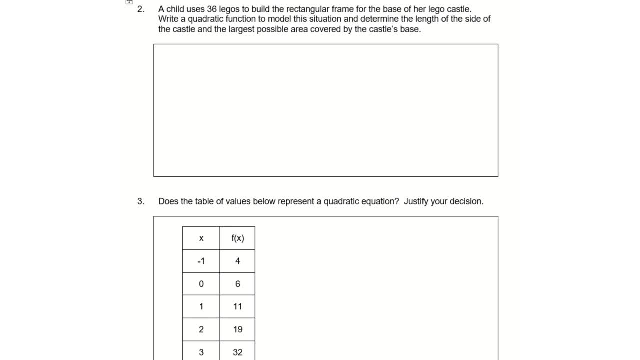 uses 36 legos to build the rectangular frame for the base of her lego castle. so rectangular frame. let's go ahead and draw ourselves a picture of this rectangular frame. so we've got a length and a width and a length and a width and we know that this. 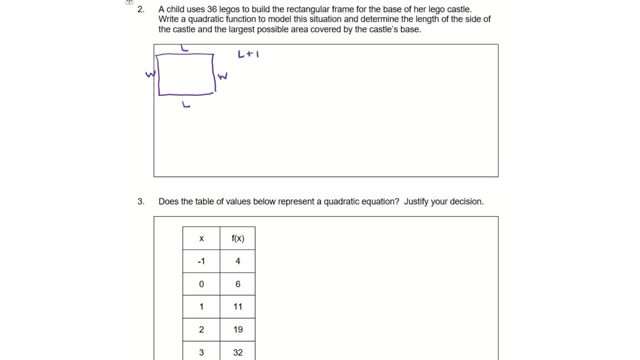 is a total of 36 legos. so length plus length plus width plus width gives me 36 legos. i can combine like terms and i can say: two times the length and two times the width will give me 36 legos, and that means that length plus width would just be 18 legos. 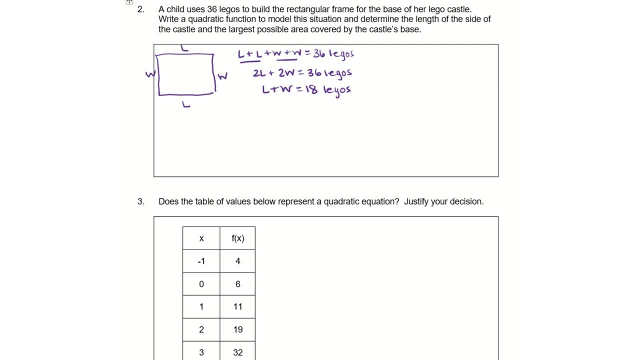 so that's a good relationship to know. we're going to keep going, write a quadratic function to model this situation and determine the length of the side of the castle and the largest possible area covered by the castle's base. so we're going to start with our. 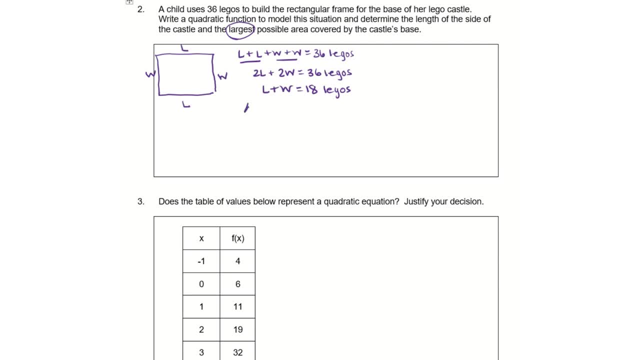 quadratic function for the area. we know area equals length times width. so if we say that the length is x, then the width would have to be 18 minus x because of this relationship, right, we know, length and width add up to 18. so if length is, 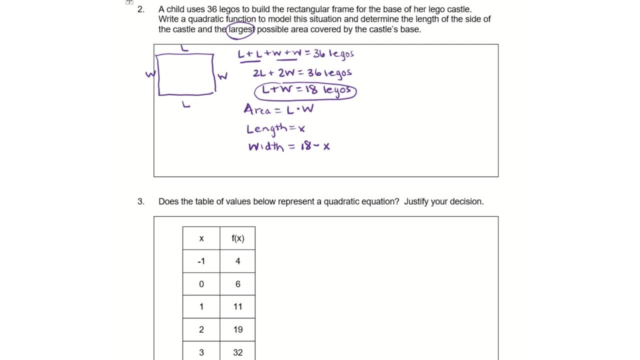 x, then width has to be 18 minus x is area equals x times 18 minus x. If I were graphing this quadratic function, my x-intercepts would be at 0, 0 and 18, 0.. Since my x-intercepts would be at 0, 0. 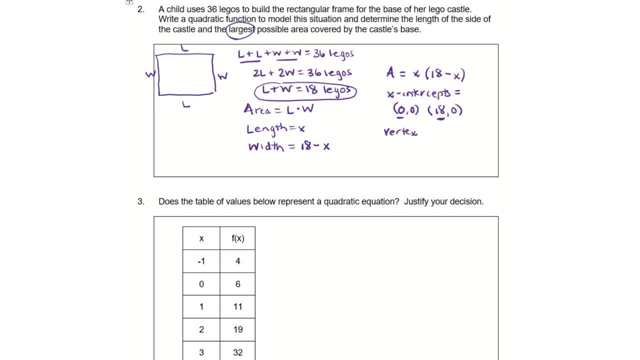 and 18, 0,. that means the vertex would happen when x equals 9, because that would be halfway in between the x-intercepts. So if the vertex happens when x equals 9,, that's when we've got the largest possible area. So the length 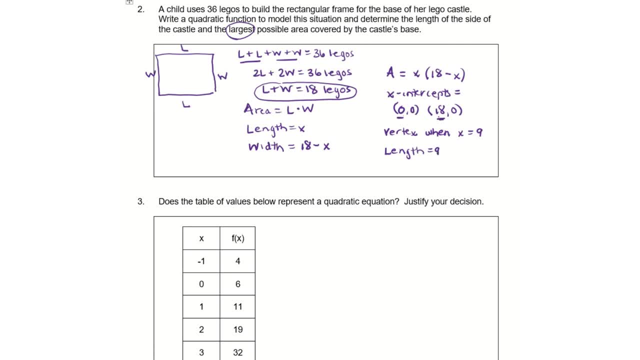 is 9,, the width is 9, because 18 minus 9 is 9, and that makes x equal to 9.. So that's when we've got the largest possible area. So the length is 9,, the width is 9, because 18 minus 9 is 9, and that makes 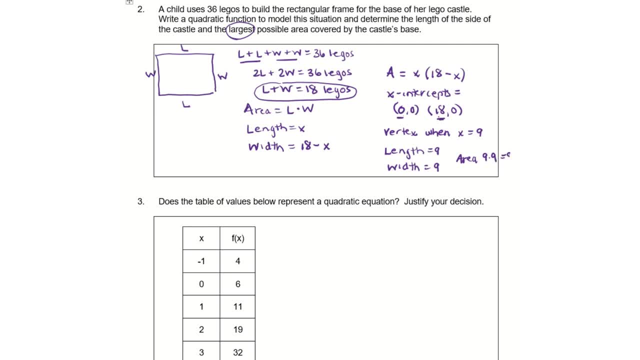 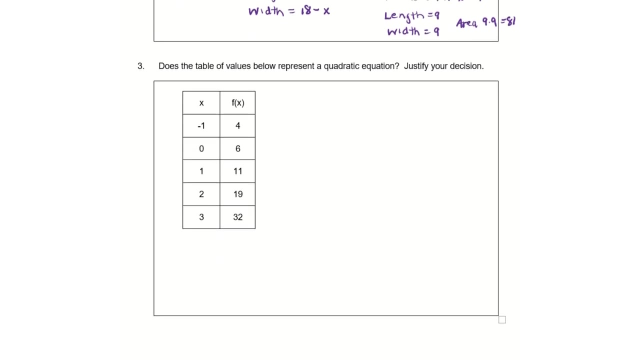 the area 9 times 9, or 81.. Alright, problem number 3.. Does the table of values below represent the quadratic equation? Justify your answer? So what we do know? I'm sure you remember that the rate of change in a quadratic function is linear. 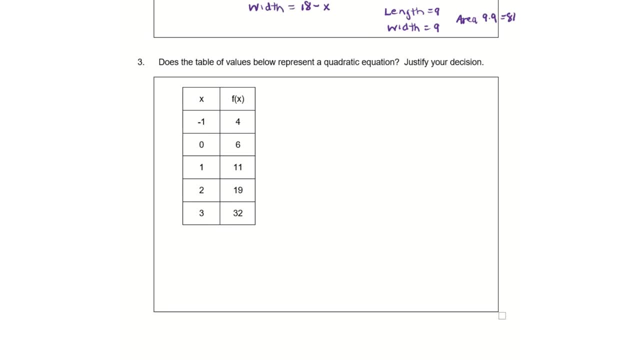 Rate of change is calculated as subtracting the y-coordinates and subtracting the x-coordinates. right? We've done that a bazillion times by now. So let's start by calculating the rate of change between the first two points. So subtract the y-coordinates and subtract the x-coordinates. 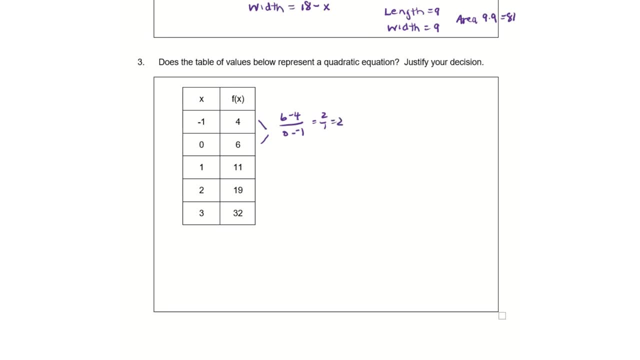 and we get 2 over 1, which is 2.. We're going to do the same thing for the next pair of points: 11 minus 6 over 1 minus 0. So that's 5 over 1, which is 5.. Do that for the next pair. 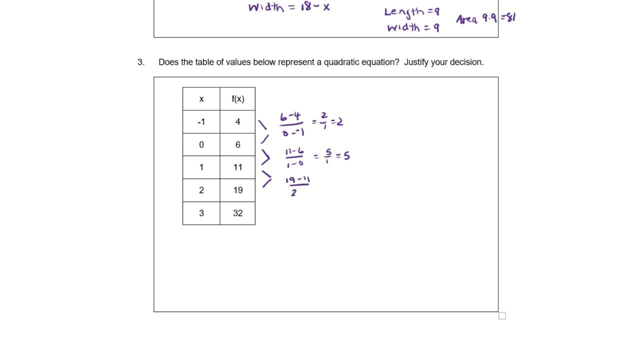 of points, So 19 minus 11 over 2 minus 1, which is 8 over 1, or 8.. And then, for the last two points, 32 minus 19 over 3 minus 2 is going to be 13 over 1,.